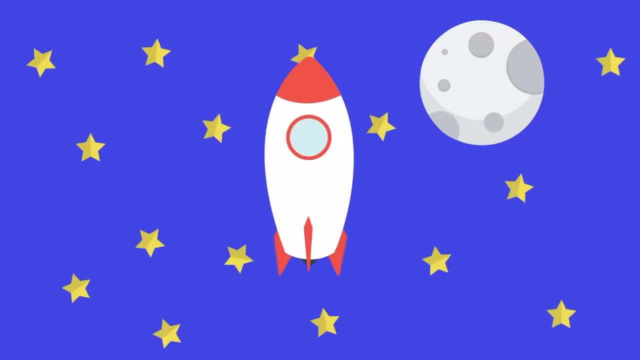 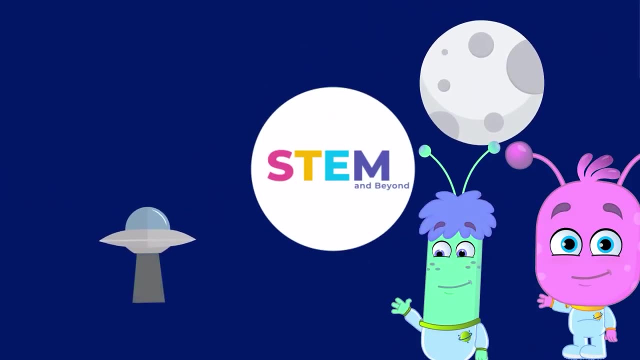 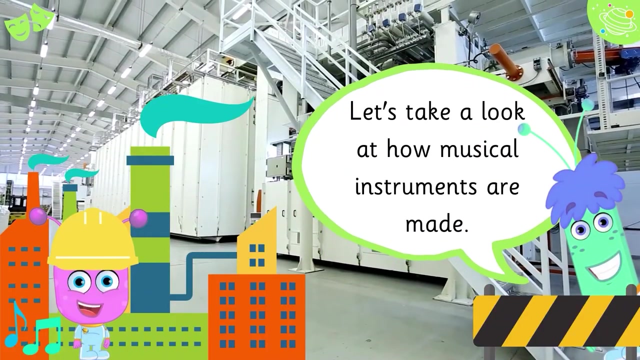 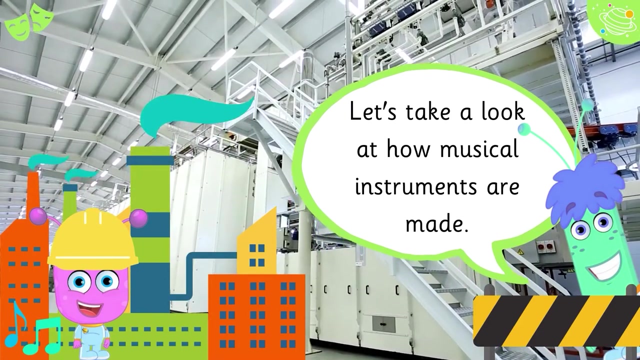 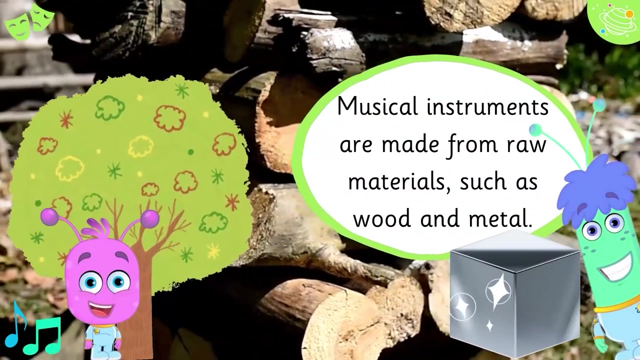 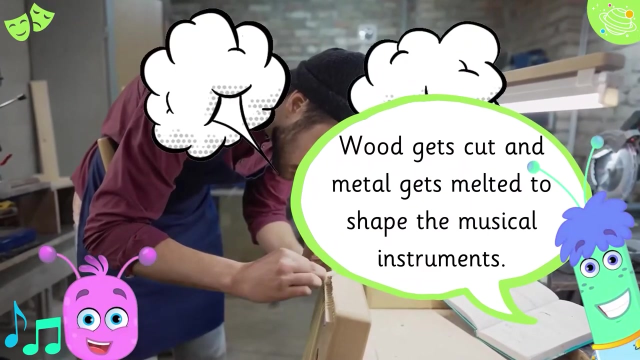 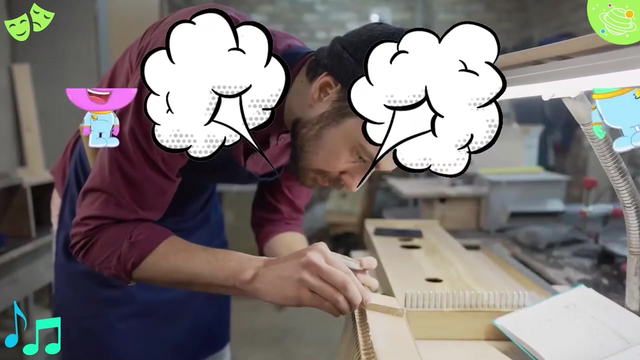 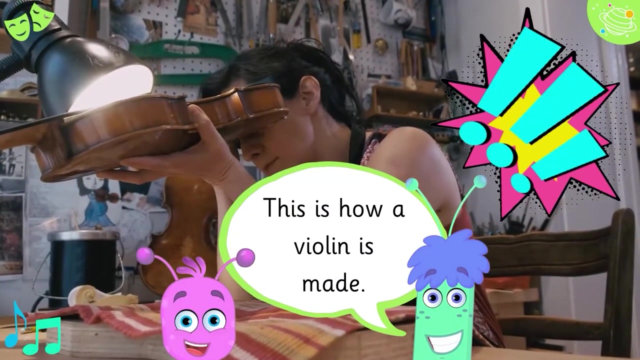 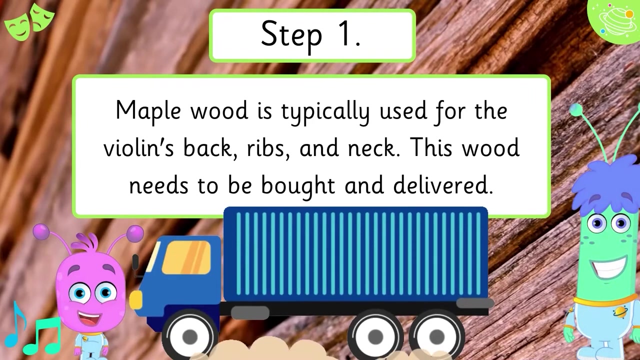 Let's take a look at how musical instruments are made. Musical instruments are made from raw materials such as wood and metal. Wood gets cut and metal gets melted to shape the musical instruments. This is how a violin is made- Step 1. Maple wood is typically used for the violin's back ribs and neck. 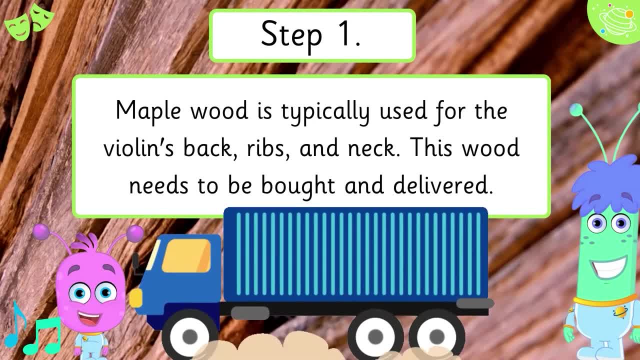 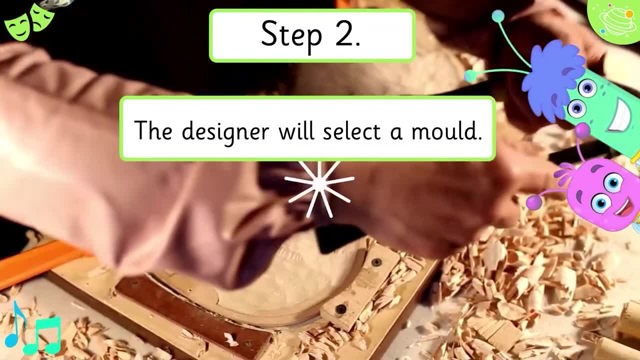 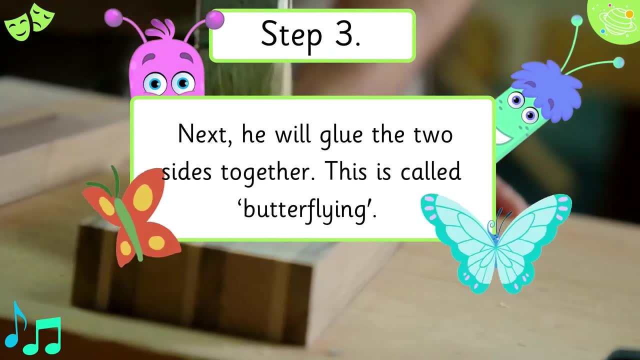 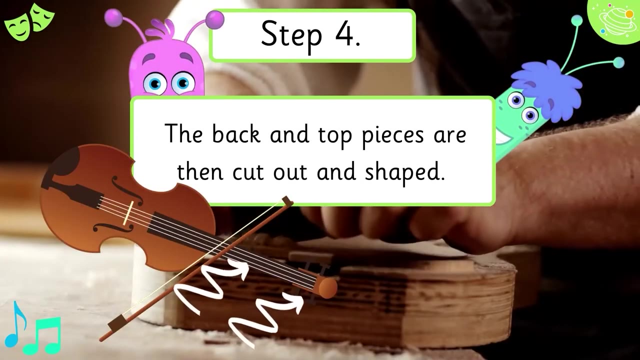 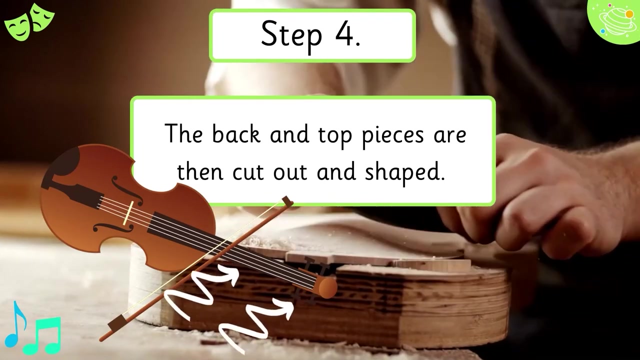 This wood needs to be bought and delivered. Step 2. The designer will select a mould. Step 3.. Next, he will glue the two sides together. This is called butterflying Step 4.. The back and top pieces are then cut out and shaped. 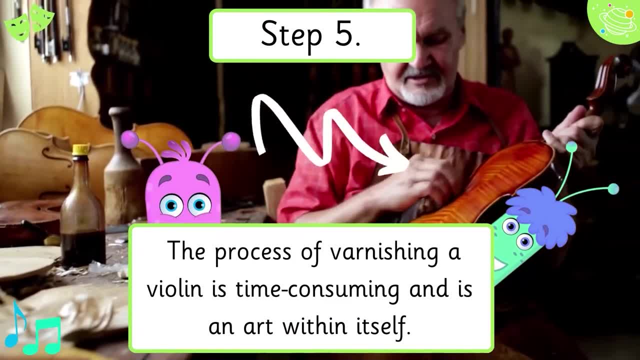 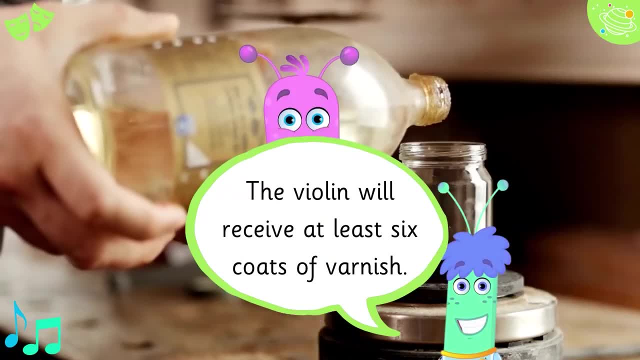 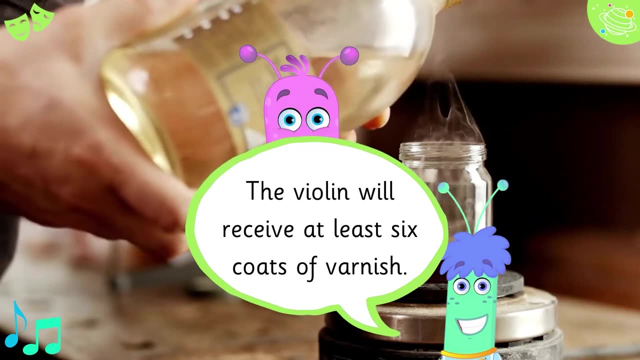 Step 5.. The process of varnishing a violin is time consuming and is an art within itself. The violin will receive at least six coats of varnish- Step 10. This will be used to make a ring. Step 11. This will be used to make a ring. 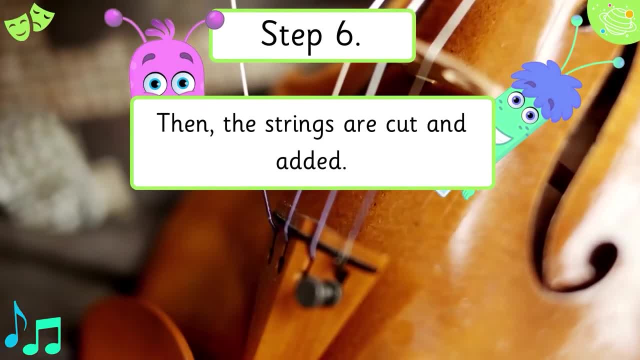 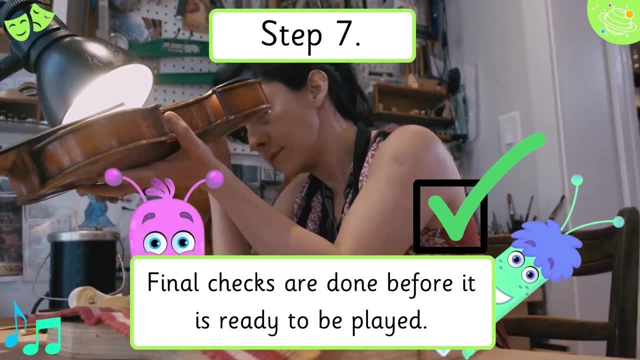 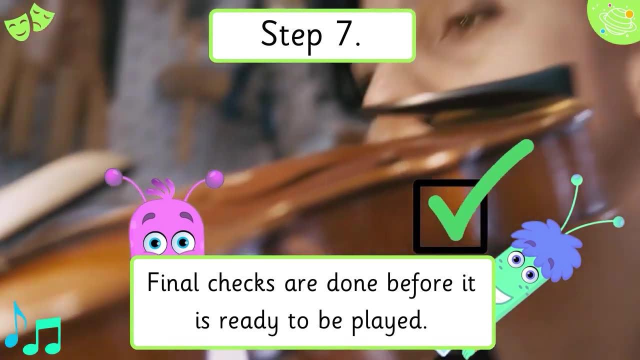 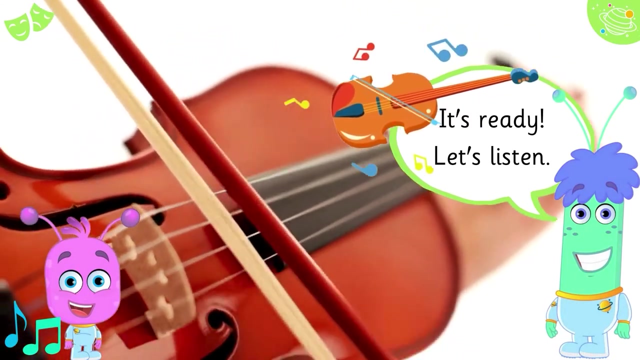 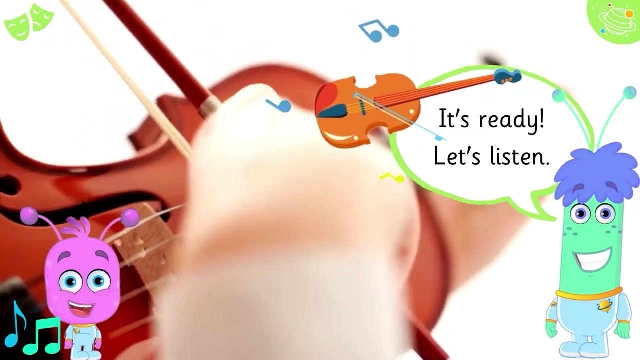 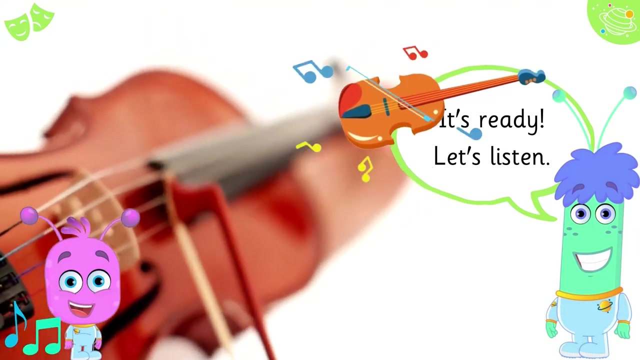 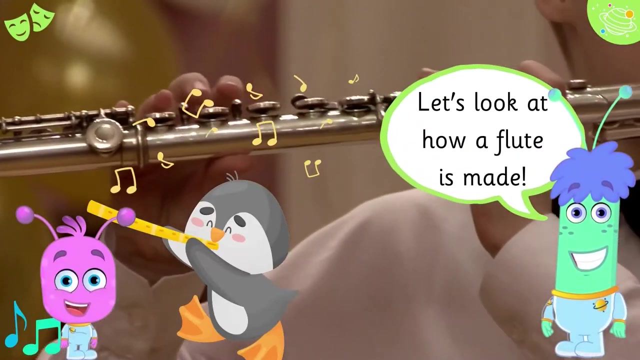 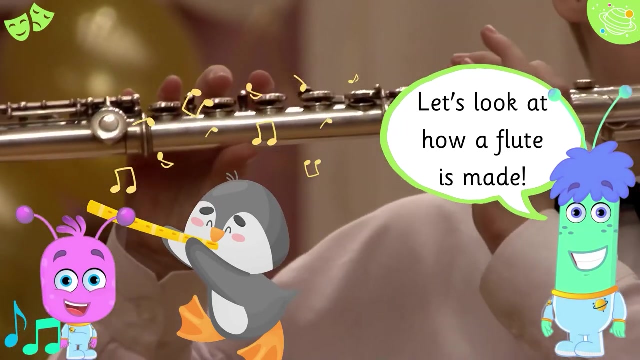 Step 6.. Then the strings are cut and added. Final checks are done before it is ready to be played in Step 7.. It's ready. Let's listen. Let's look at how a flute is made. Flute makers need to do 5 years of training.